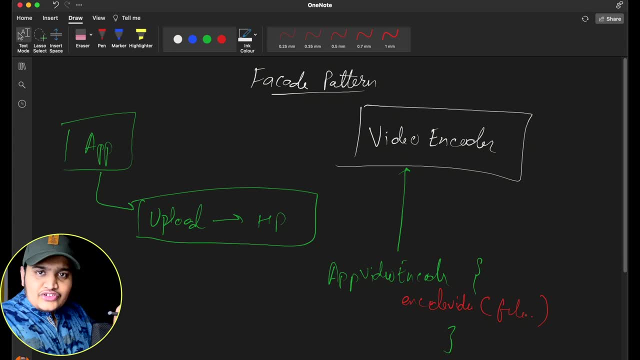 video. So you can see that we are just adding one abstraction layer and that abstraction layer will help us to reduce a lot of complexities of the other framework or a library that we want to use. So whenever you have a scenario where you want to reduce the friction, to use the other. 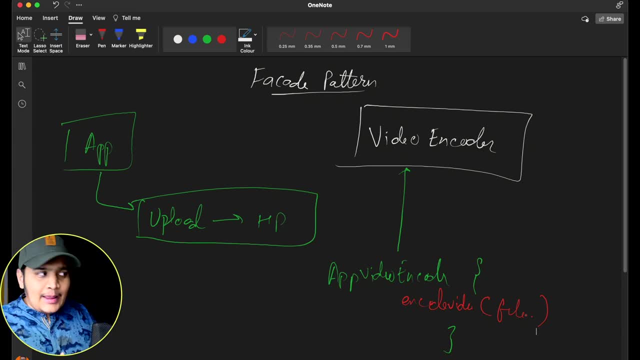 library or to have the abstraction on top of that particular library. At that time we will use the facade design pattern. So this type of pattern is widely used in the industry. We might be using it, but we might not know as well, because we generally do a lot of things. 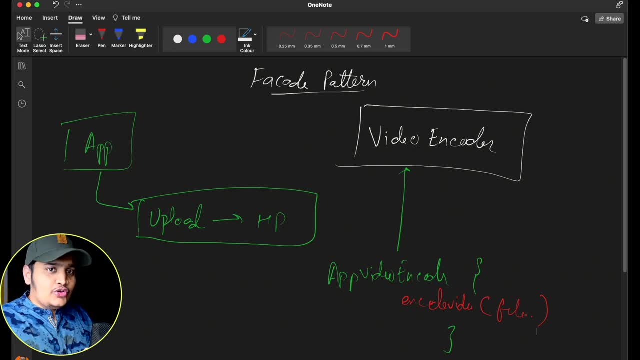 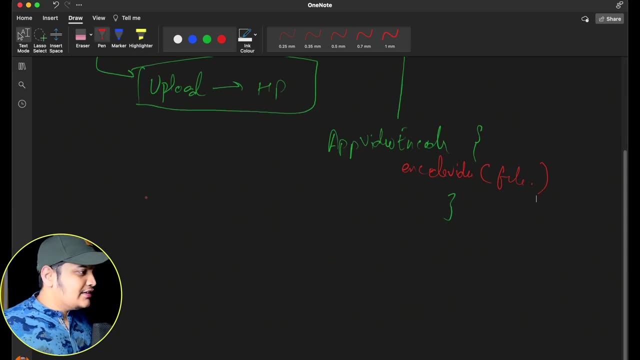 We create an abstraction on top of the other libraries that we want to use, and at that time it is easy for us to implement that as well. So that's called a facade design pattern. Let's take one more example here. Suppose we have the Zomato store. okay, So Zomato is. 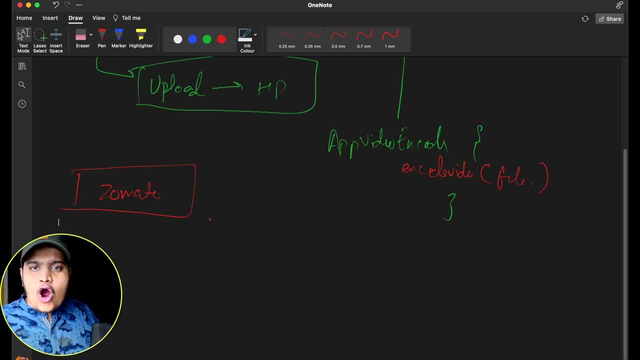 a food delivery app. okay, With the Zomato service, we can order the food and a delivery person or a delivery partner will get a food from the restaurant and it will deliver to us. So you can see that ideally you are ordering a food from the restaurant, but here Zomato. 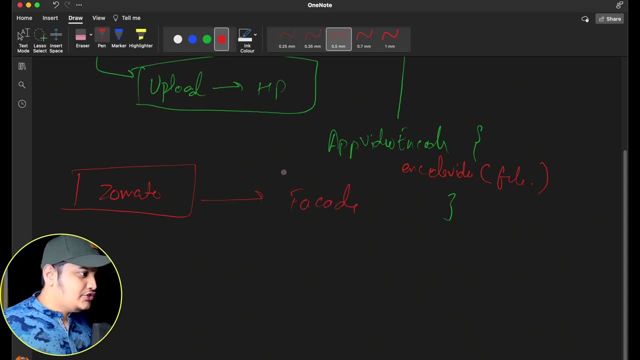 is your facade in between, okay, which will help us to order a particular food from the restaurant, and a delivery partner will take that food for us and it will deliver us. So here you can see that Zomato is responsible. It's the abstraction where it will help us. 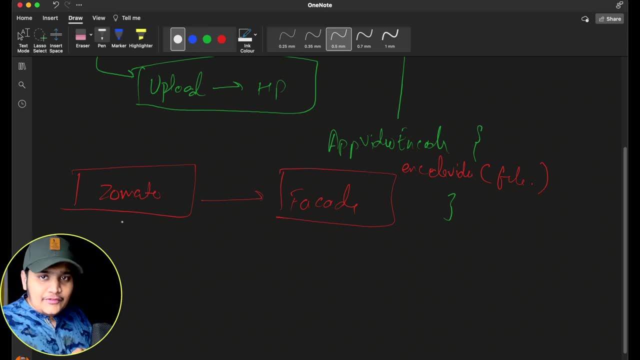 to do a lot of process. It will help us to order food. It will also intimidate the restaurant that you need to prepare this food. It will assign a delivery partner as well, and delivery partner will get that particular food delivered to us. So a lot of things happening and you can see that there are a lot of things involved. 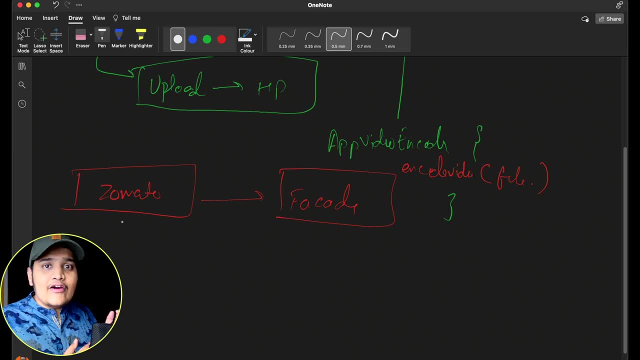 as well, but Zomato will have the abstraction and it will simplify everything for us to order food. So that's how facade will help us. So let's take the same example- the Zomato delivery app example- and see within the code as well. It's really going to be very easy. 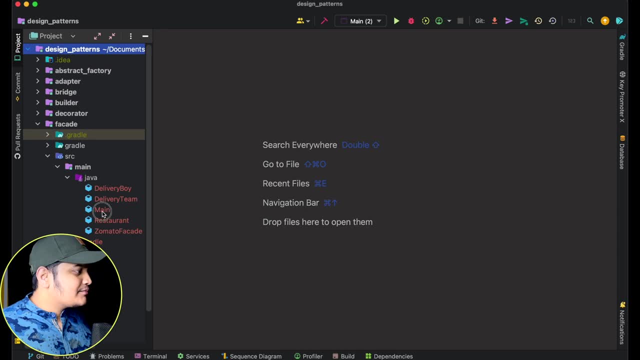 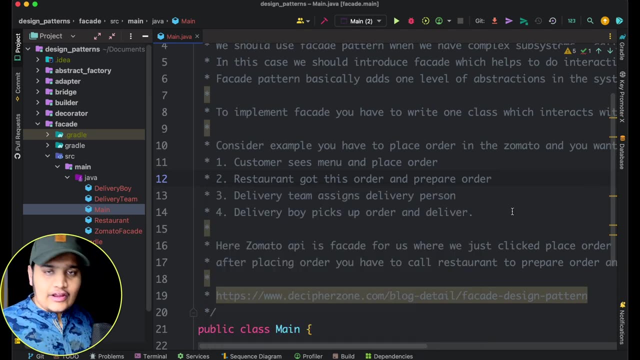 Okay, you can see that I have the facade design pattern here and I have the main class. if you want to go to the theory part, I have added the theory as well and I have added all the information from where I have taken the references as well. So all the information you will get. 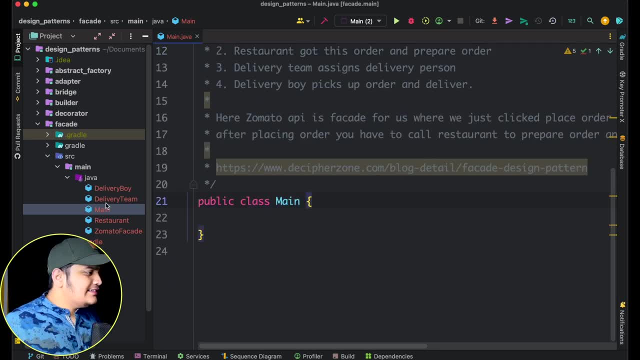 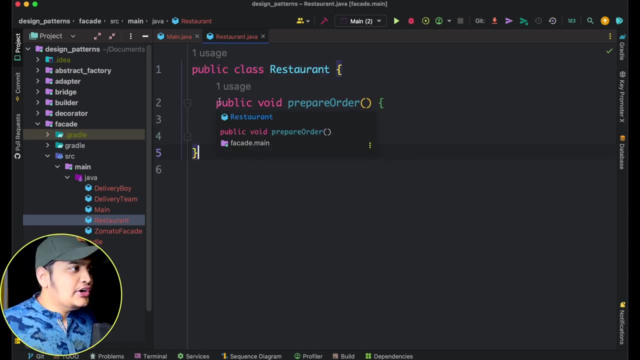 from here. I will add the link in the description below for you to check. Now you can see that I have the restaurant class available here. Okay, so you can see this is a restaurant class and this restaurant class is responsible to prepare my order. Okay, so that's one thing.